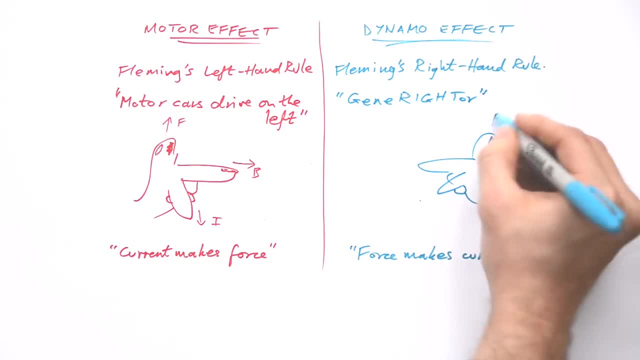 So it's exactly the same, With thumb being the thrust, first finger being the field and second finger being the current. So that's how we remember which one we're supposed to use. Fleming's left-hand rule for the motor effect: Motor cars drive on the left. Fleming's right-hand rule used for generators: Generator. 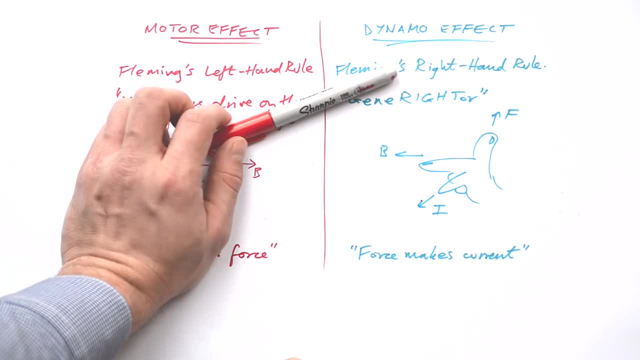 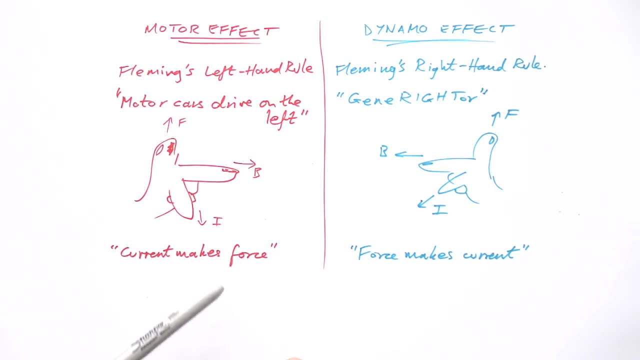 the dynamo effect. So we do have a problem with this then, don't we? Because if we have a current going through a piece of wire and that's causing it to go downwards, then we're getting a current to make a force. But the problem is that we don't have a current going through a piece of wire and 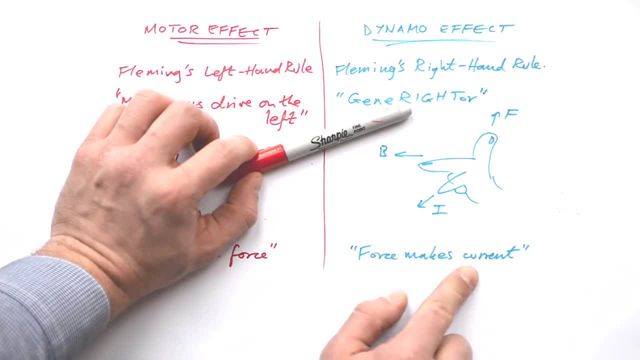 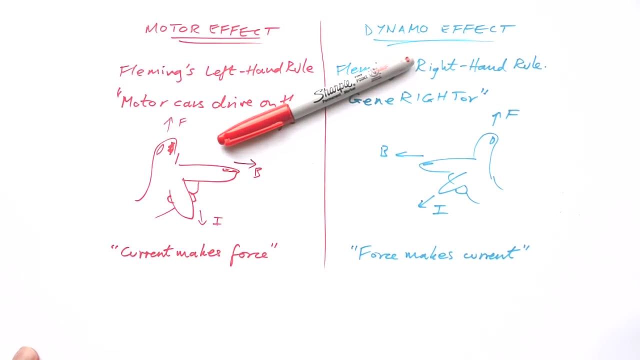 that's causing it to go downwards, then we're getting a current to make a force, But the problem with that, then, is that we have a force and that force in turn makes a current as well. So it seems like we cannot have one without the other, and that's absolutely true. 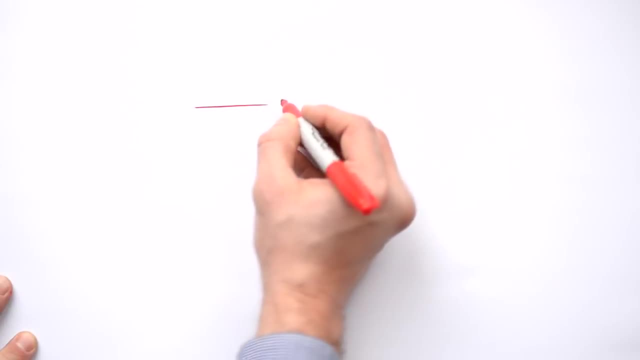 But it does make sense if we think about it. Let's go back to our magnets, with a wire in between, So north, this is our south, So that means our magnetic field is going in this direction. We have a wire that is part of a circuit going through here. 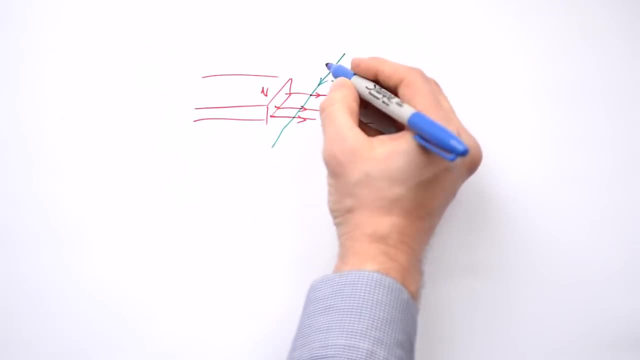 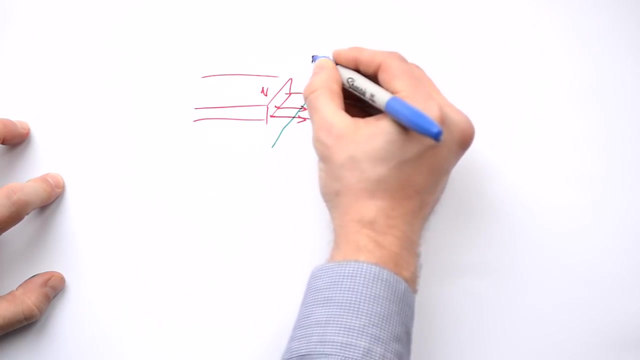 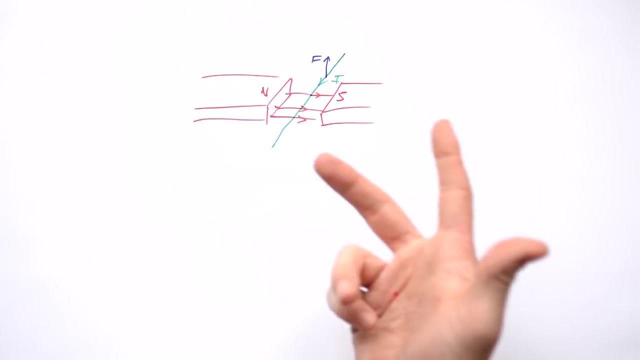 and we have a current going in that direction. So that is going to produce, according to Fleming's left-hand rule, a force going upwards, But also. so now we have a wire moving through a magnetic field, We now actually have the dynamo. 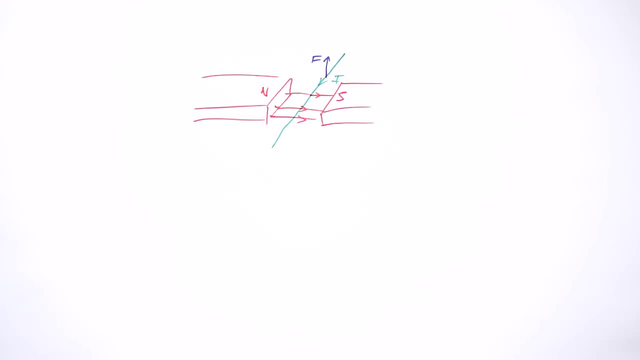 effect as well. So now we have to bring in Fleming's right-hand rule. Our field is going to the right, We have a force going upwards, So that actually means that we have our second finger going back up the other way. So what happens? Dynamo effect tries to stop the motor effect. 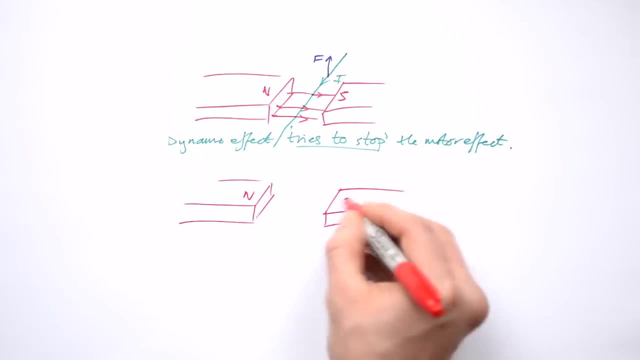 It also goes the other way around as well. Let's say we're starting with a wire and we actually force it downwards. Let's get our Fleming's right-hand rule. So field's going that way, Force is going downwards. Our current 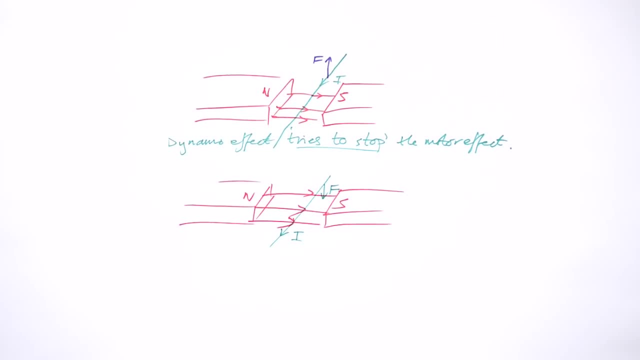 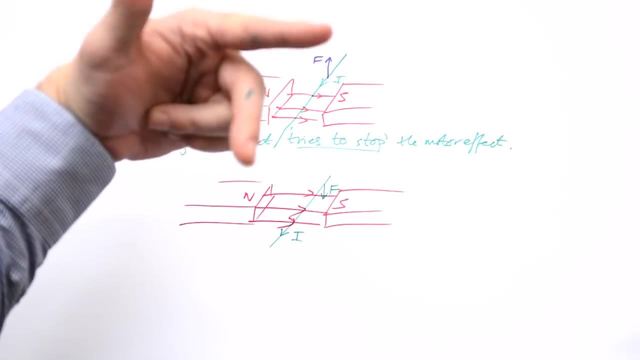 is going to be going in this direction here. But the problem is now is we have a current going through a piece of wire, So we now have to bring in Fleming's left-hand rule. Let's just check it: Field's going that way, Current's going that way. We're actually producing a force. 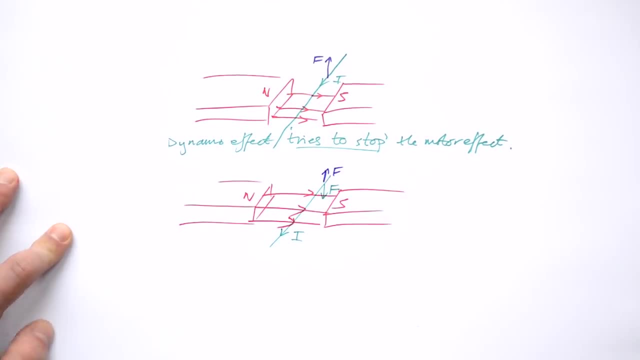 going in the opposite direction. So once again, the motor effect tries to stop the dynamo effect. We basically just arrived using that idea and that's what we're going to do. So we're going to apply Lenz's law. That is the direction of an. 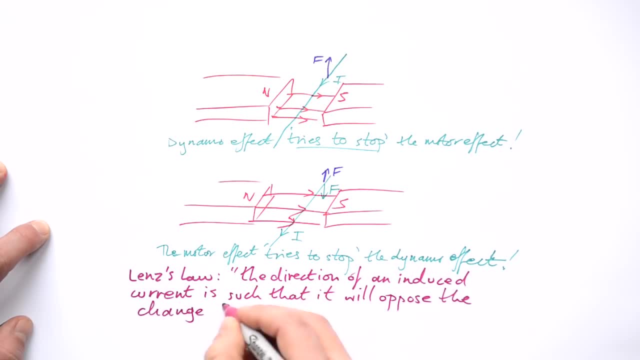 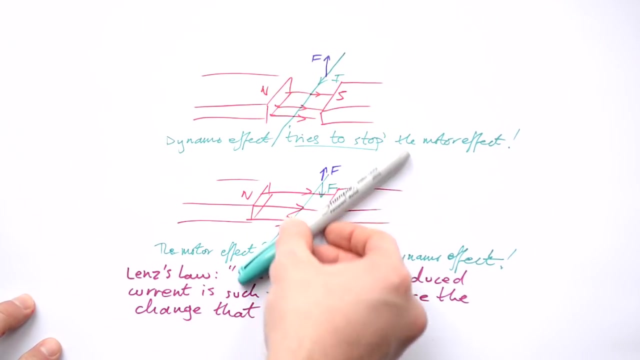 induced current is such that it will oppose the change that caused it. So let's just apply Lenz's law to this situation. here We have our wire that we're pushing downwards and that's producing a current in the wire, But that current in the wire in turn, 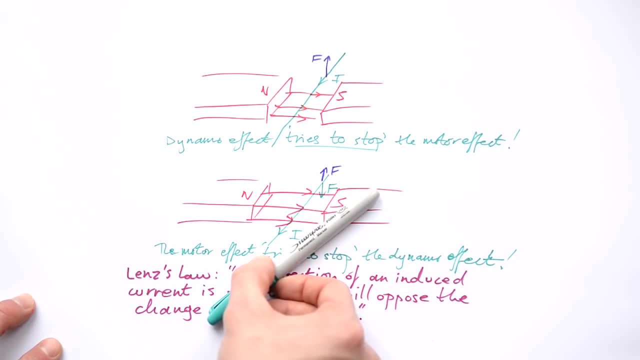 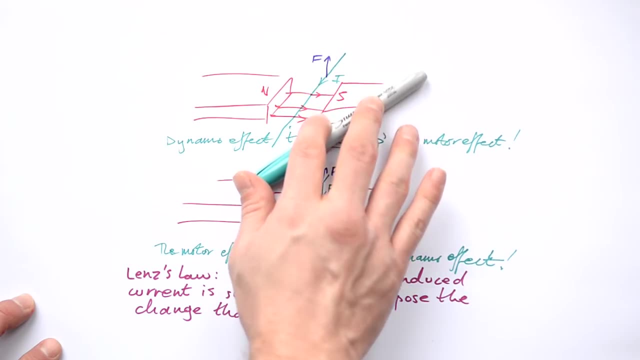 is going to be equal, and opposite force that's going to try and push it back upwards. What do we see happening? These two forces are equal. If we apply a force on a piece of wire through a magnetic field, it effectively reaches terminal velocity Because the reaction force 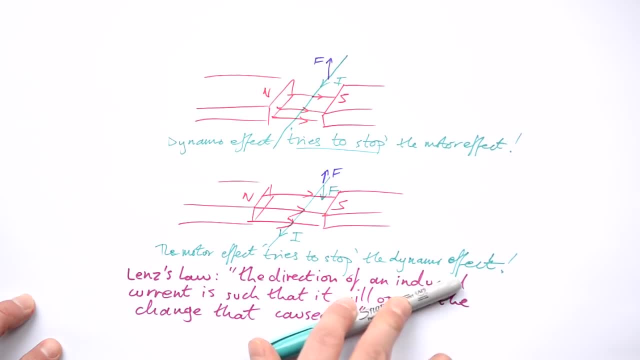 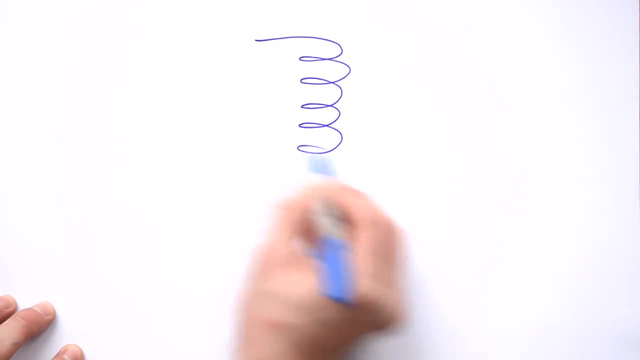 due to the motor effect is going to be equal to the force that we're applying to begin with. There's no better example of Lenz's law than when we have a coil of wire, that is, a solenoid, as part of a circuit. 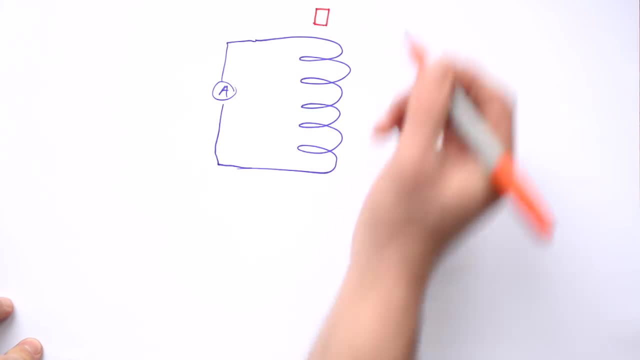 So let's draw a magnet and we drop it through this solenoid. This magnet has its own permanent magnetic field. Now we could draw some field lines on there. What happens? as this magnet falls through, The flux of the magnet cuts, as it were. it crosses the wire, It crosses the solenoid as it. 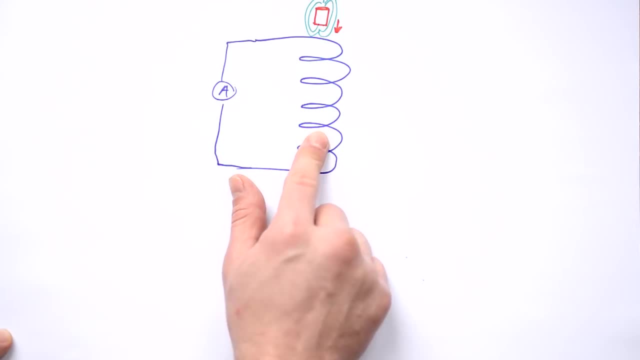 goes down As the flux passes through or cuts the wire. or we can say the other way around, that the wire is cutting through the flux. doesn't matter which way around it is, this wire experiences a change in flux, So we are going to. 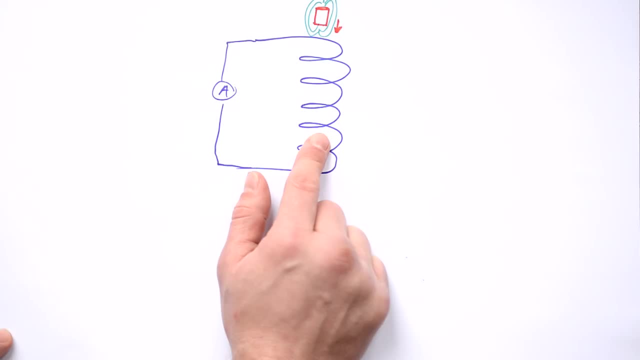 have a current being induced in this wire, The electrons are going to move. Now we're dropping it in north end first. Now let's just have a think about this logically. This magnet falls through. As it cuts the wire, it produces a current, It induces a current in the wire. That 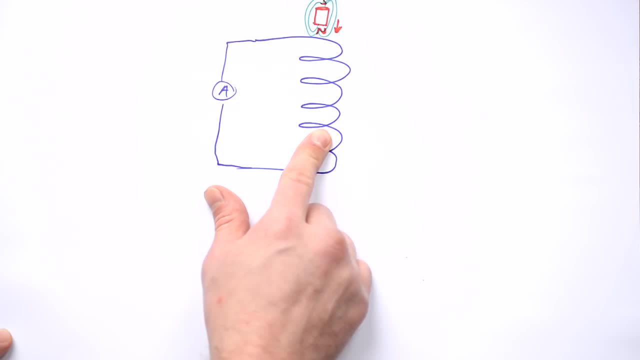 produces its own magnetic field as well, And the question is which end of the solenoid is going to be the temporary magnetic field? north pole and south pole? Let's have a think about it If you have a magnet going in and we have a south pole being induced in the solenoid at the top. 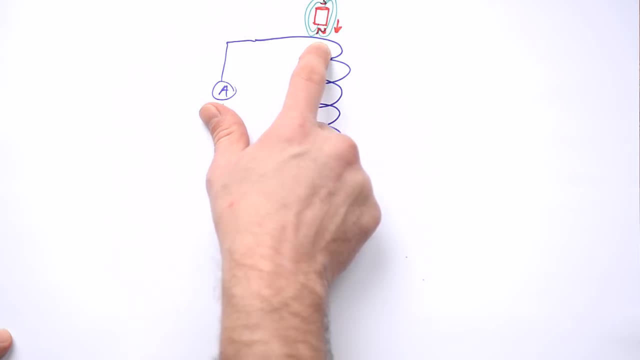 we know that north pole and south pole attract each other. What's going to happen? The magnet is going to speed up. As it speeds up what happens? The magnetic field produced by the current in the wire gets stronger and it attracts it even more. So if it was a south pole being, 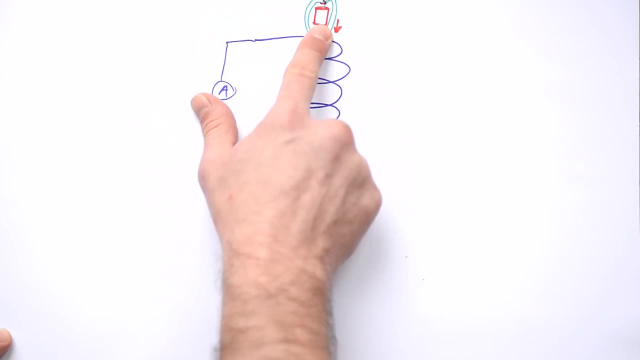 induced at the top here to begin with, then that would mean that this magnet would accelerate faster and faster and faster, and it would just go like that. So we're in effect getting energy for nothing. But we know due to Lenz's law that whatever current is induced, it will try. 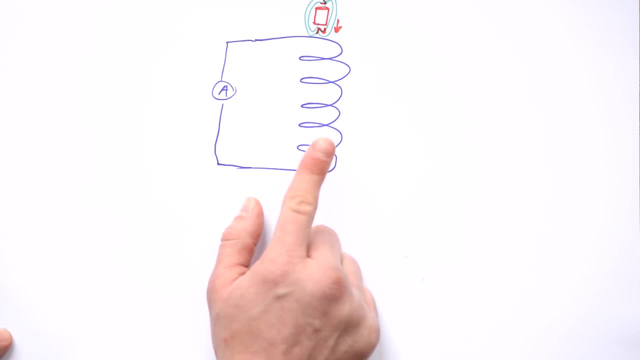 and stop the change that caused it to begin with. So what makes more sense then? If the north pole comes in, we actually have a north pole being induced at the top. Therefore, we have a south pole at the bottom. Just one thing that's useful to know. 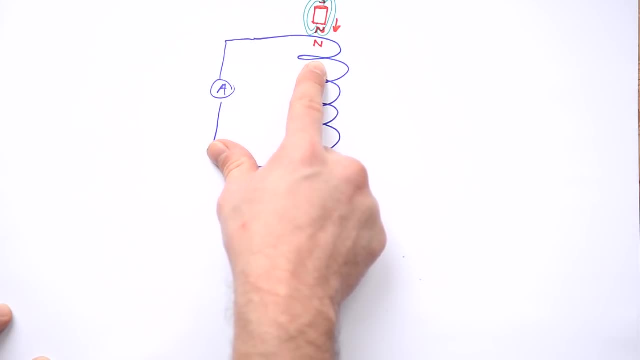 how can we tell which way the current is being induced in this solenoid here? Well, if we look from above a little eye and we're looking down on this solenoid here, we can say that if you have a north pole, then the ends of that end- if you put arrows on the end- are going. 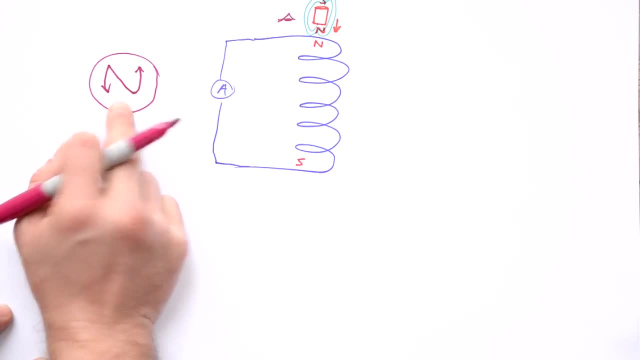 anti-clockwise. So if you have a north pole induced at the top and we're looking down, then that means our current is going to be going anti-clockwise. What about from the bottom? Well, if we draw an S and put arrows on the end of that S, we see that the arrows are actually going. 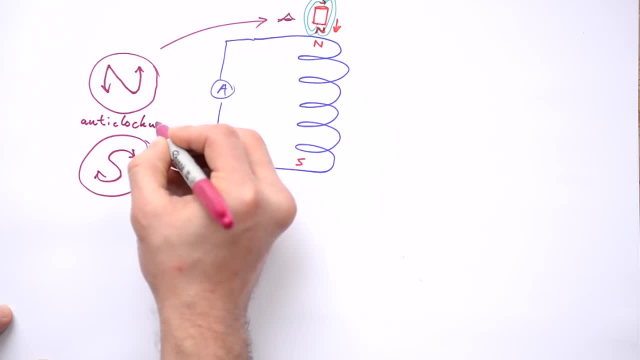 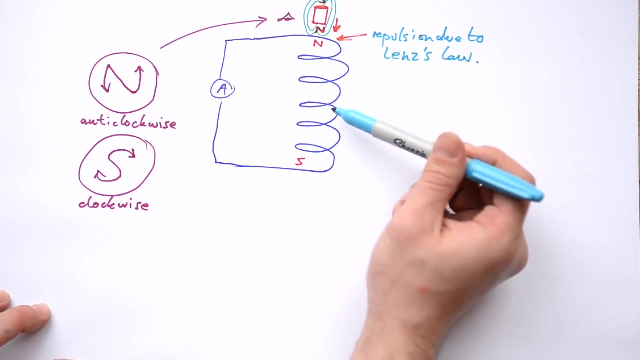 clockwise. So that's how we can predict what direction the current goes in when induced in a solenoid. So what happens if you have a north pole being induced at the top of our solenoid? that means that we have repulsion and that's due to Lenz's law, In other words, the solenoid. 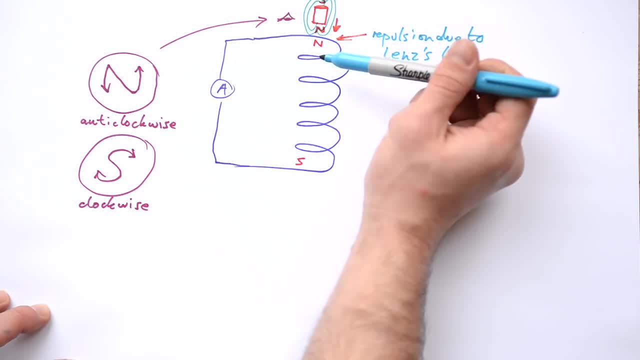 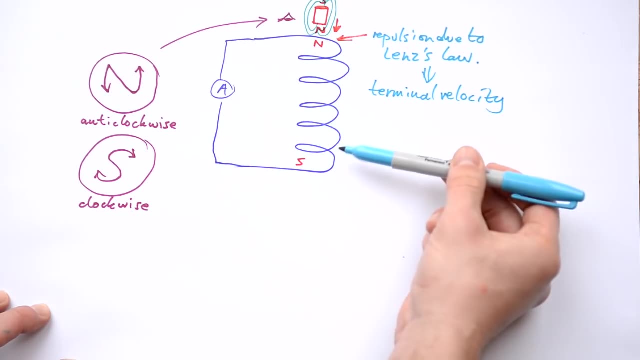 doesn't want the magnet to enter it, so it's trying to stop it. So what happens? It actually reaches terminal velocity. As one of these magnets falls through this solenoid, it actually produces a force that is equal and opposite to the magnet's weight and it falls at a terminal velocity. 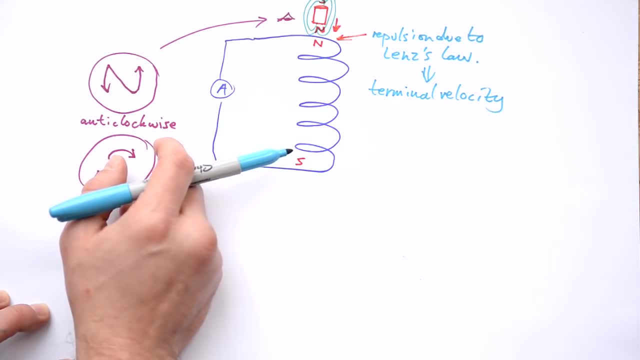 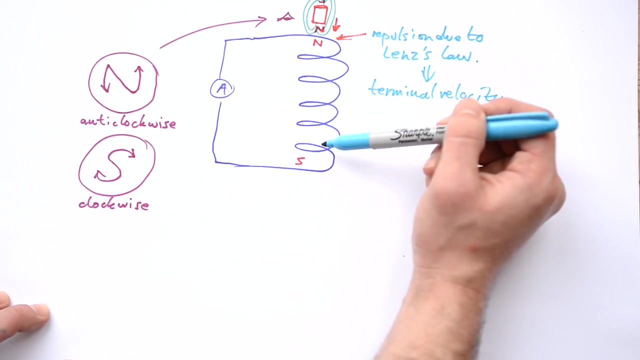 This is the same for a solenoid, and it also works for just a pipe as well, which you can think of as an infinite number of these little loops going down. If that's the case, then we need to have energy lost somewhere, And whether it's a solenoid or a pipe, ultimately energy gets lost as heat. 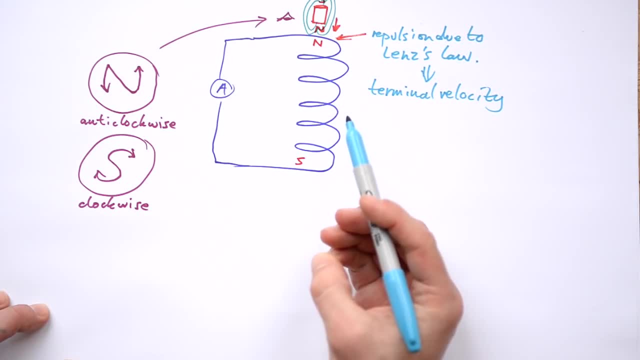 as we have a current setup here and we have energy dissipated as heat due to the resistance. Hang about, though, Once our magnets actually exited the solenoid. if we still have a south pole here on our solenoid, doesn't that mean that the south pole 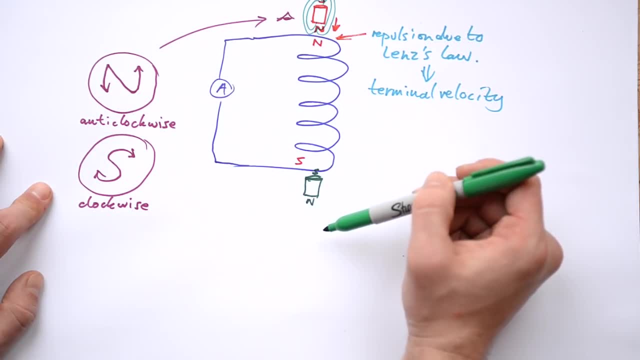 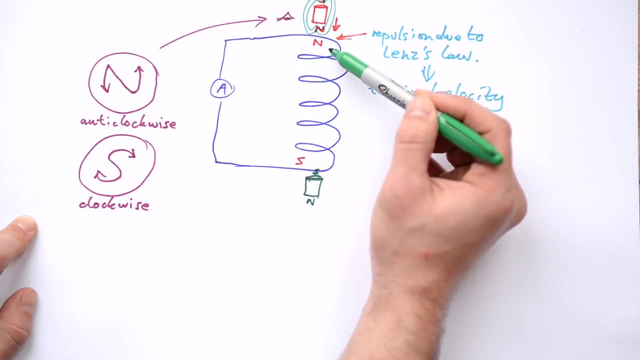 is going to repel the south pole of the magnet and it's going to push it away and accelerate it. Well, we know that can't be the case. due to Lenz's law. The coil of wire tries to stop the magnet from coming in by producing an equal and opposite force, but the weird thing is is on the way out. 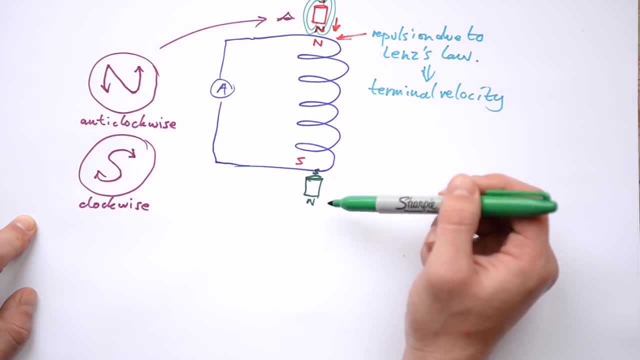 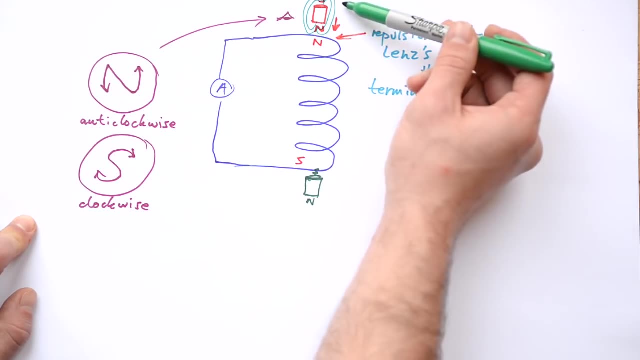 the coil of wire tries to stop it from leaving. In other words, Lenz's law means that magnets and wires always want what they can't have. The coil of wire doesn't want the magnet to come in, but once it's in it doesn't want it to leave. That must mean that on the way out we have attraction. 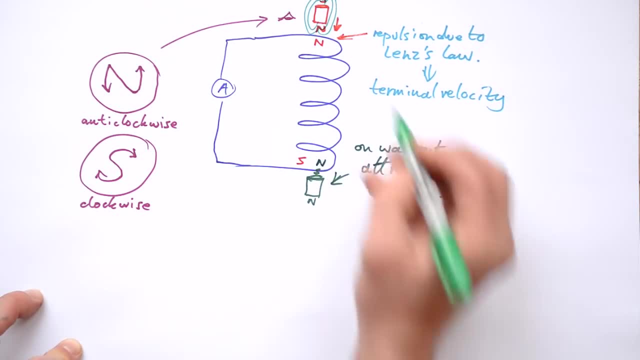 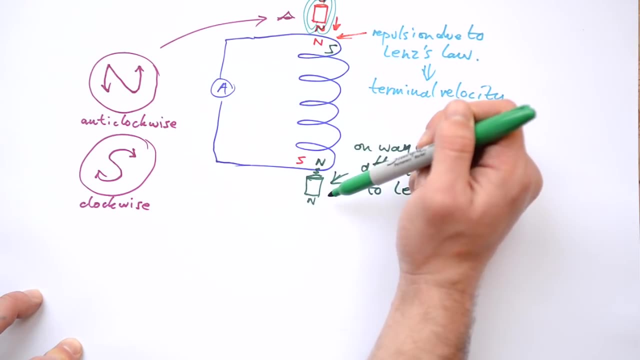 due to Lenz's law. So we have to have a north pole at the bottom of our solenoid now and a south pole at the top. What does that mean? Well, that means that between the magnet entering the coil and exiting the coil, we actually have a complete flip of magnetic field induced in this coil of wire. 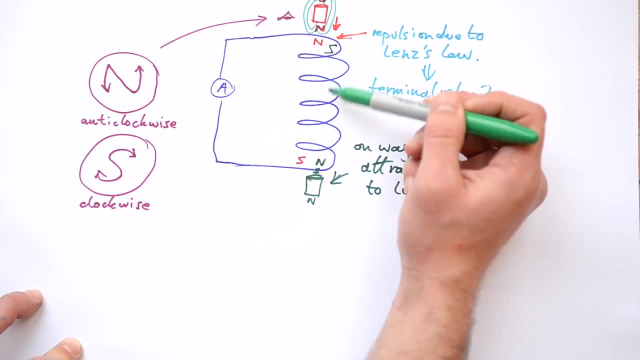 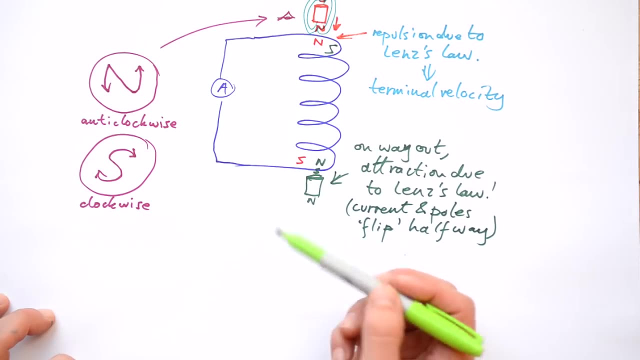 That must mean that the current starts going one way but then halfway through it flips and starts going the other way. So we have a complete flip of magnetic field induced in this coil of wire The other way. So Lenz's law, we know, is the direction of the induced current is such that